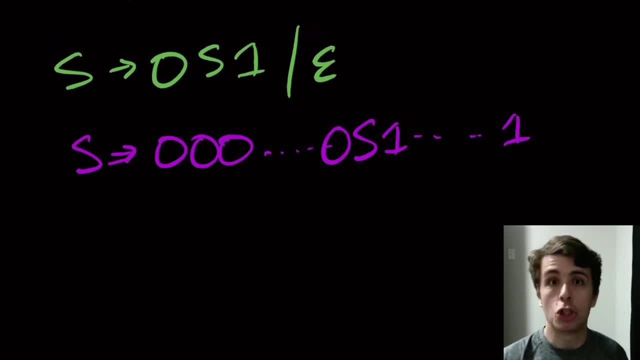 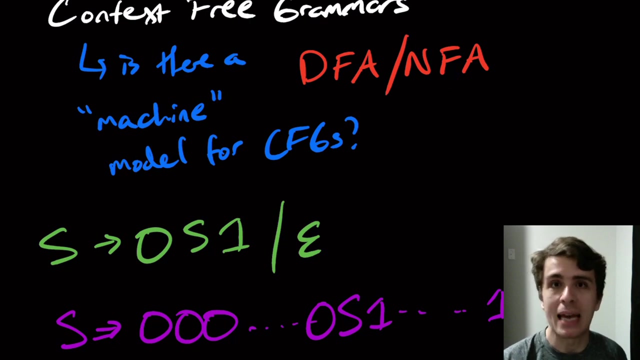 things right. So if we want to have a machine model for the context-free languages, we need to be able to input a string and say yes or no onto it. Well, clearly we need something more powerful than a DFA or NFA, which means we can't just have states and transitions and whatnot. We've got to. 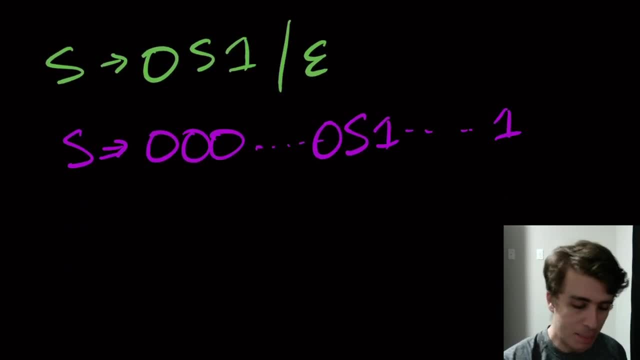 have something additionally to this. So let's think about what's happening here. So let's think about what's happening here. Well, these, eventually we're going to have a string of 0s, then a string of 1s, right, Because we're going to apply this first rule until we're done. 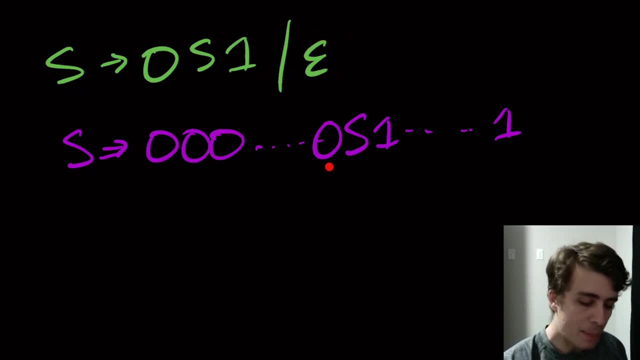 and then we apply this one, of course. So what happens here is these 0s at the front. if we think about it, there's no variable that occurs in there And consequently there's no variable in this particular case. But no matter what either, a variable. 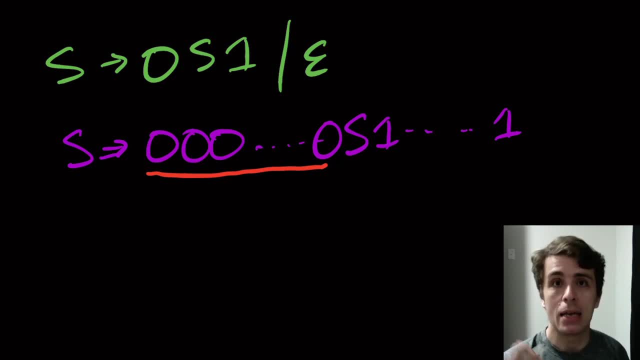 is going to appear first or a terminal appears first, right. So remember, if a terminal appears first, it's never going to change. So if we want to have a machine model, what we can do is we can simulate a rule application, And if a terminal appears, then now what we can do is: 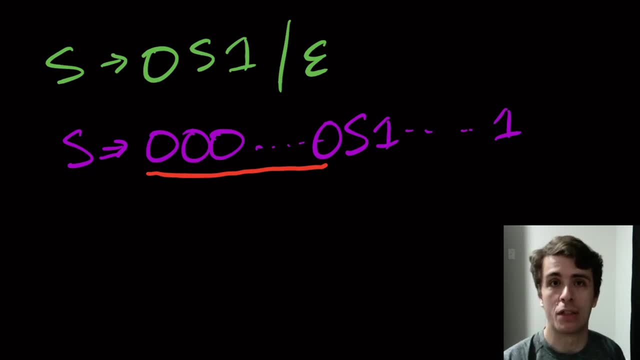 read that corresponding character off of the input. So in this case, when we apply this rule right here, this 0 is never going to be modified at any point because it's a context-free grammar. So then when we have the string as input, we will read the 0s off of read a 0 off the input. 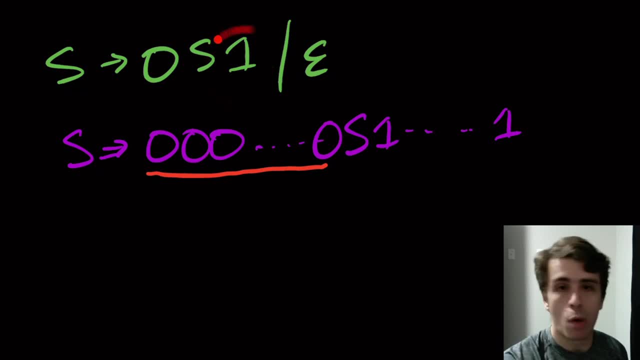 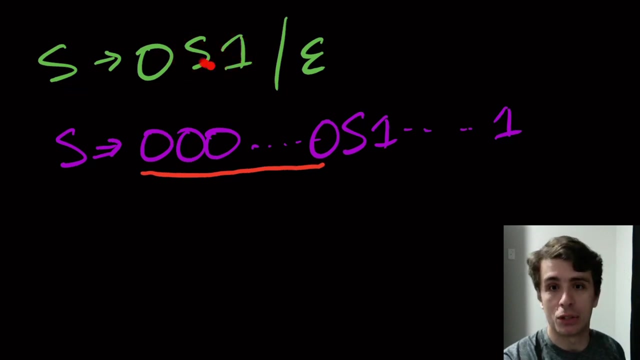 because it's right at the front. This 1 won't be read until later, because this s in the middle could theoretically produce anything right. So what we want to do, then, is we could have a whole load of these variables and a whole bunch of stuff on the right here. So, from this s onward, 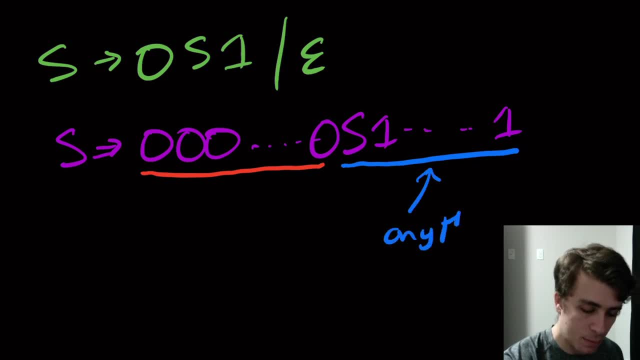 this over here can be anything. right, It could theoretically be anything, But we know that this is only terminals And we can deal with those by reading off of the input the same thing that was produced by the grammar, But over here it could be theoretically anything. So what we would need? 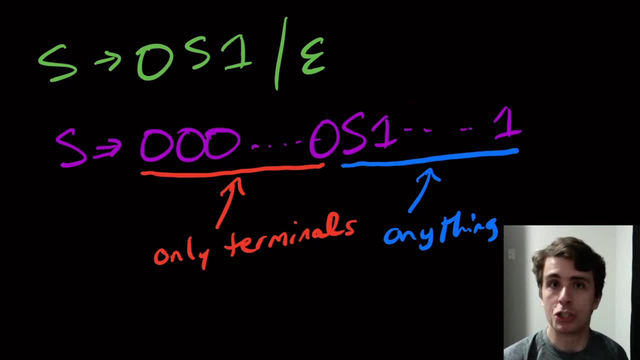 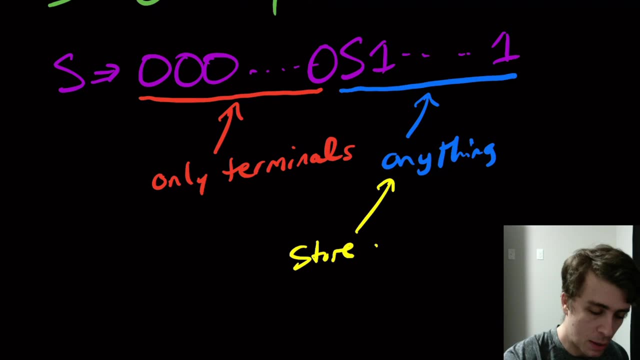 to do is to store all that stuff onto some structure. So that's what we're going to try to do. So what we need to do is to store all this somehow. Well, we can't store them in states, because this right-hand side could grow as long as we need to Think about this. If we look at 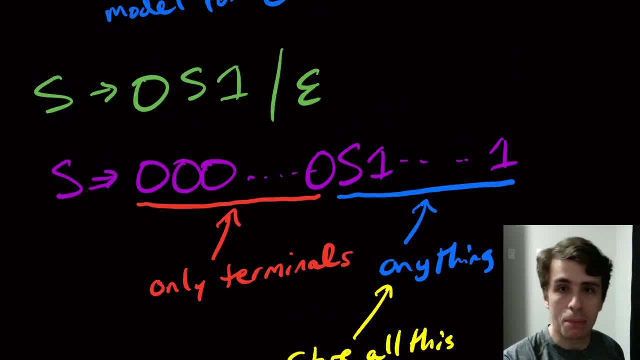 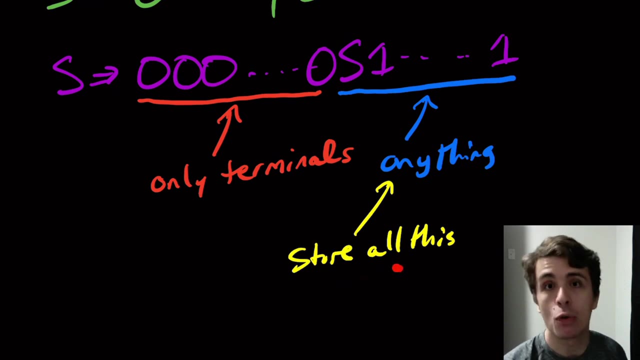 this right here. the number of ones that we produce by applying this rule over and over and over this could grow arbitrarily big. If we had some limit, we can surpass that limit no matter what. So if I tried to bake this into the states, I'm going to have trouble. So what we need to do is 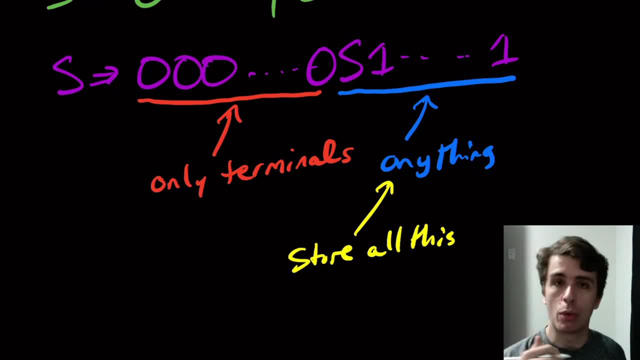 to have some kind of structure that grows, right. So we need to have some kind of structure that grows and is not fixed like the states are. Another thing that we should notice is that we can always use a leftmost derivation. So, remember, we can always use a leftmost derivation Because, remember, it's a context-free grammar. 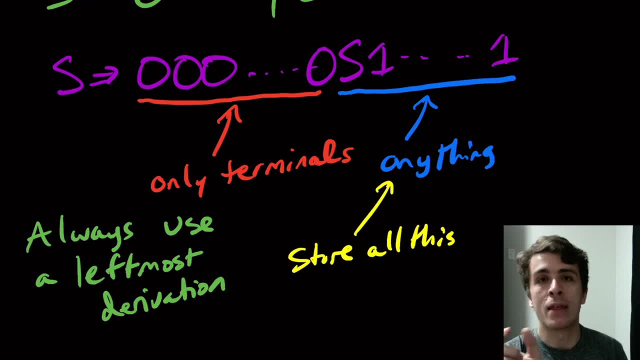 if we have a bunch of variables that we could apply a rule with, we can always choose the first one, the leftmost one. So that indicates here, because the string is being read from left to right and we can always use the leftmost one. we can always use the leftmost one, So that's. 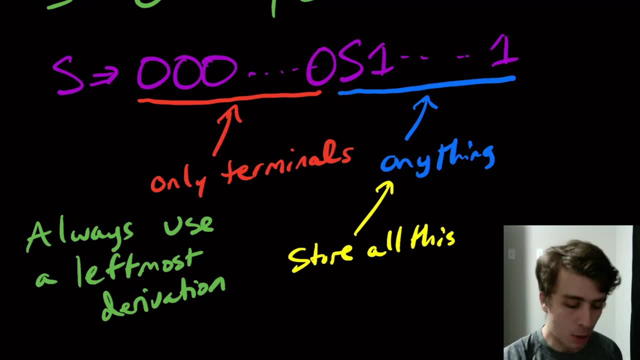 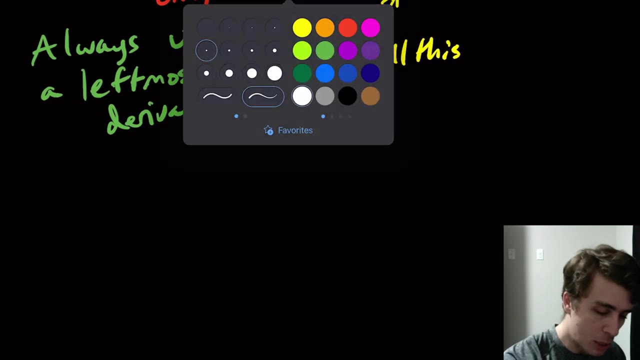 variable without changing the language of the grammar. This tells us we need some kind of structure where we can access stuff on one side, And that is the motivation for using a stack. So the machine that we're going to be talking about from a few videos from now on is something 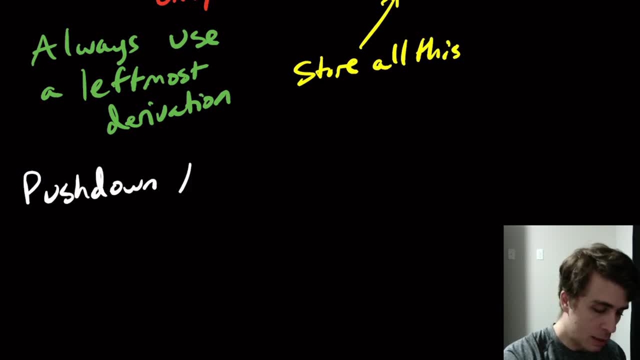 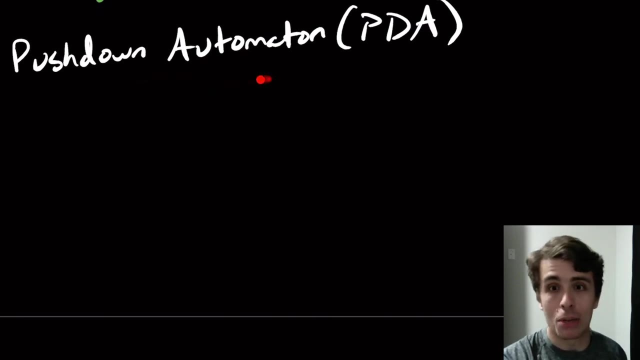 called a pushdown automaton And it's abbreviated PD, Not public display of affection, Although you may want to talk about that more than this, probably. But yeah, these are called pushdown automata And they're exactly the same. 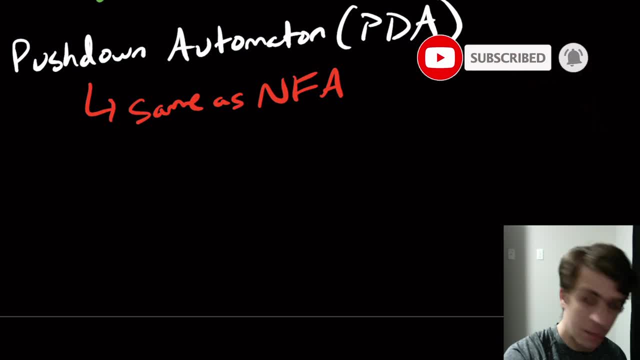 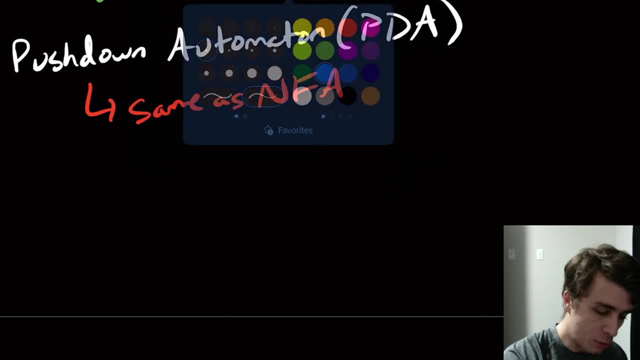 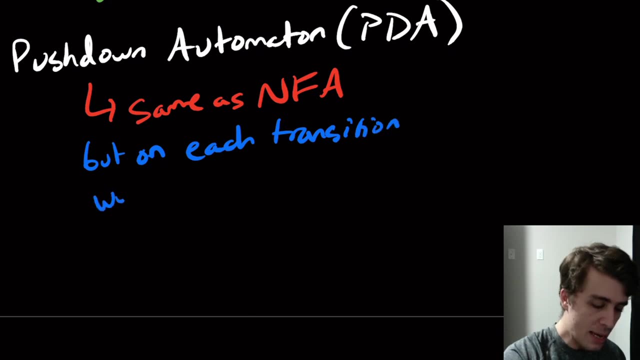 as an NFA. except now we're going to have an additional thing built into the transitions. So but on each transition we we can push or not. We could not push onto a stack. We could pop or not onto the stack. 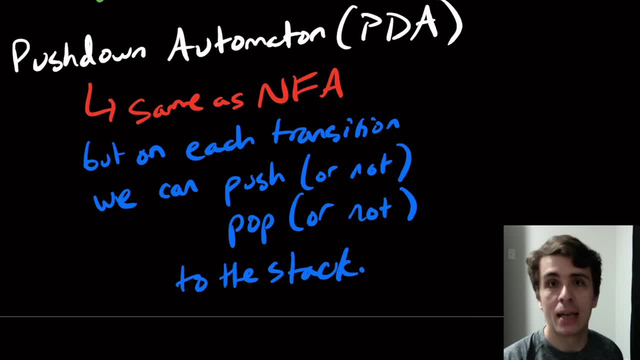 So we're only going to allow ourselves one stack, And I want you to think about why we're only going to restrict ourselves to one. If we have two, it actually changes the model, but we're going to stick with one because it's simpler. 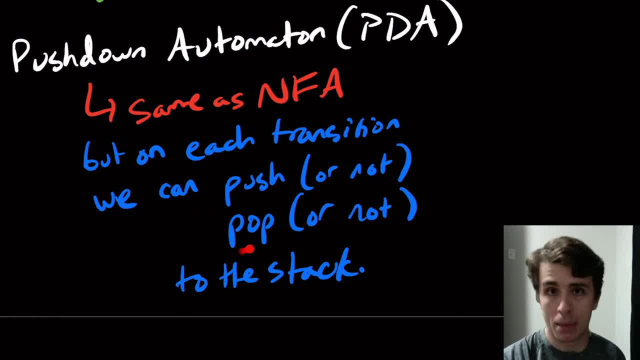 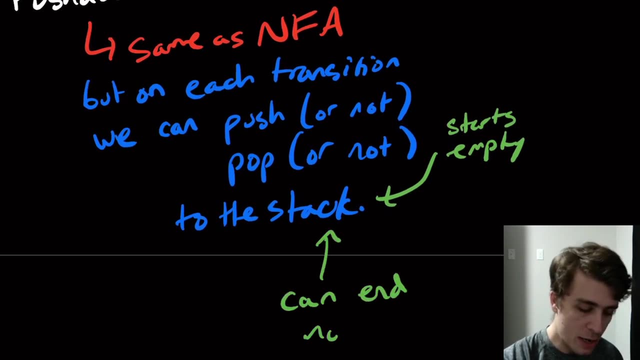 So we can push onto the stack or we can pop to the stack. Some properties of this stack are that it starts empty And another one is that it can end non-empty. So when we're all done and we accept or whatever, we don't have to have an empty stack. We could, if we want to and there is a way to enforce it. 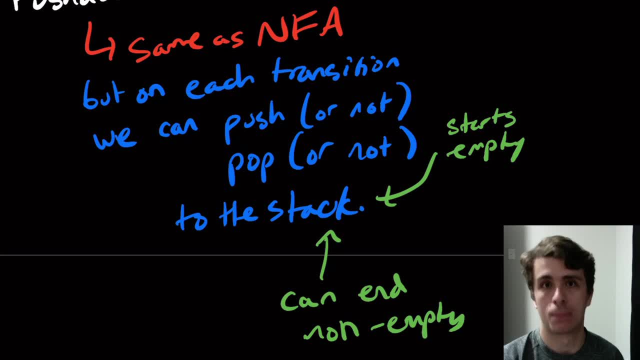 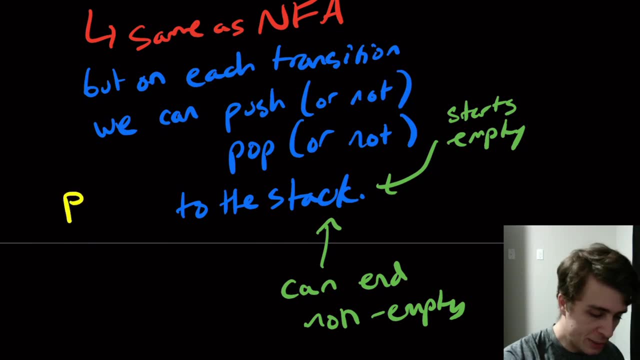 but we're we are not going to require ourselves to do so. Okay, So how are the transitions going to look? So we're going to have have transitions that look like this: So let's say, state P to state Q. 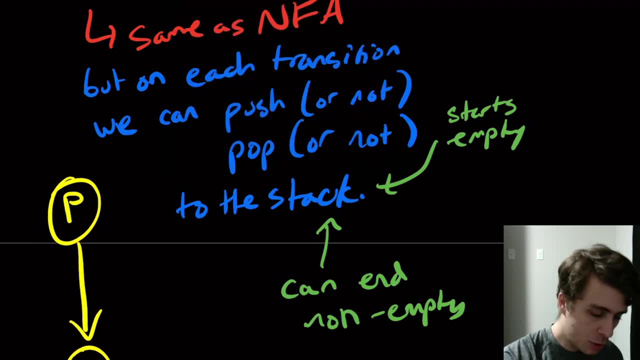 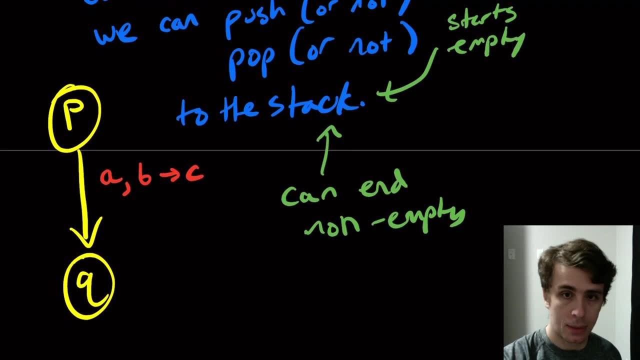 So here's what the transition is going to look like. It's going to look something like this: A, comma, B, arrow, C, And what each of these mean. the A here means what we read, So that's what we read. The B here is what we pop. 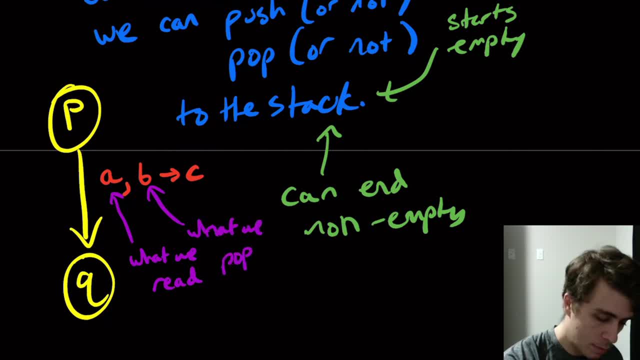 And the C here is what we push. Actually, I'm just going to simplify this to say what read: pop, push, And there's a very good reason why it's in this order. So the read has nothing to do with the push or pop, because 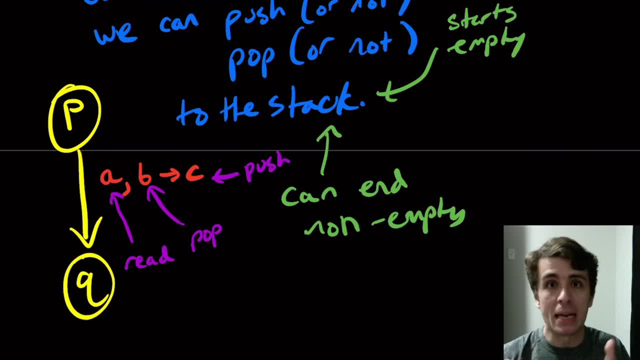 um, the reading has not, is just coming from the input. It has nothing to do with the stack. So we could theoretically put anything we want onto the stack, regardless of what's being read. Um, oh, another thing. we can only push or pop one thing at a time, or zero. 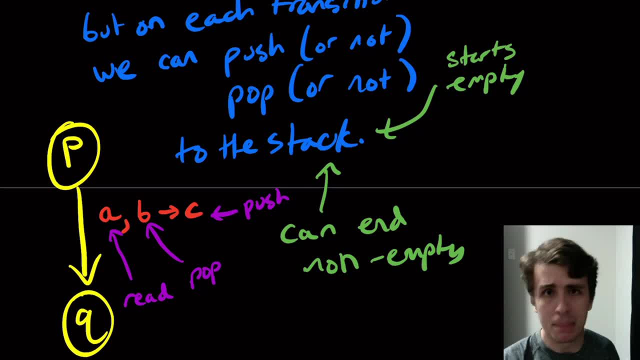 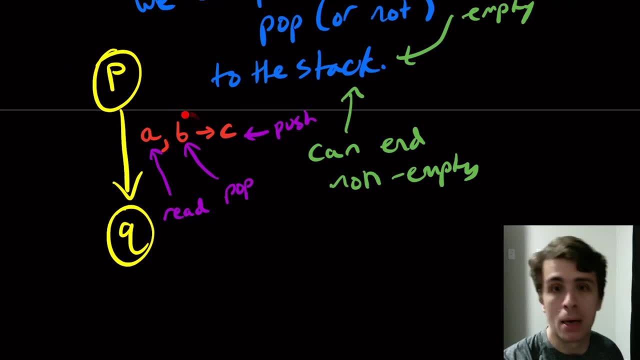 We could ignore pushing or popping, So that'd be zero. Or we can push one character on at a time, or pop, So it's important that the pop appear first, and we can only take this so that. here's something I should also note. 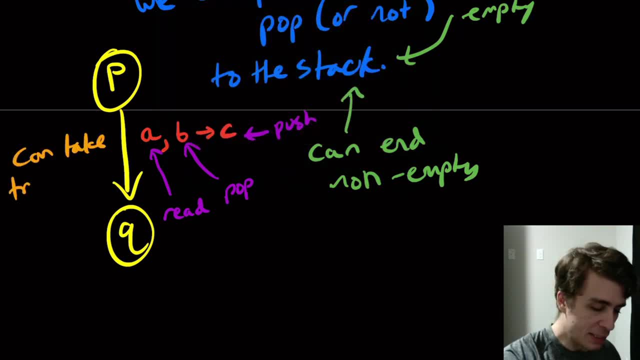 So we can, we can take the transition, We're allowed to take it. if, uh, we can read the A and note that the A here could represent a character or empty- It doesn't have to be a character. And two, we can pop the B. 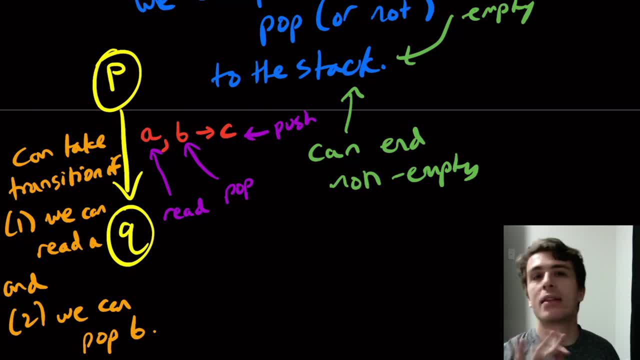 So if we fail either one of those, we're not allowed to take the transition at all. So think about it: If we can't read something there's no, we can't take the transition, just like with the NFA, DFA type model. 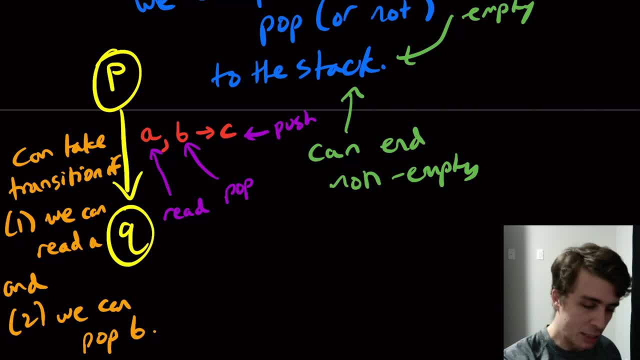 But if we can't, if we want to take this transition but we can't pop this, then that means that we're trying to pop something that's not on the top of the stack and which doesn't make sense, But with a stack. 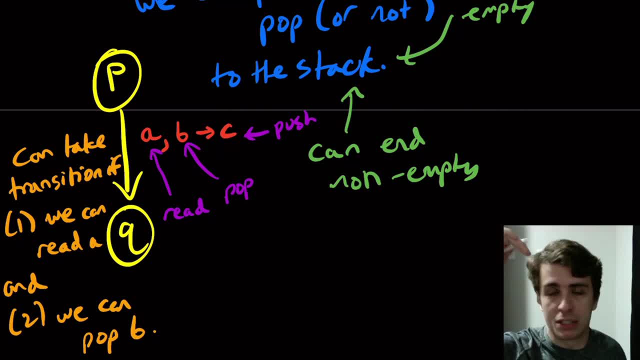 you can always push stuff onto the stack regardless what's what's there, because we're just pushing on one side. So we that's why the pop appears first, because if I'm doing a pop and a push at the same time, 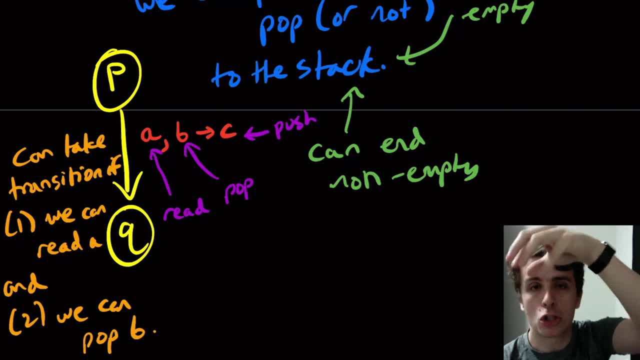 if I did the push first, then I'm just going to push a character on, But the thing I want to pop is not at the top of the stack anymore. It's below whatever I just put on. So that's why we have to pop first and then do the push. 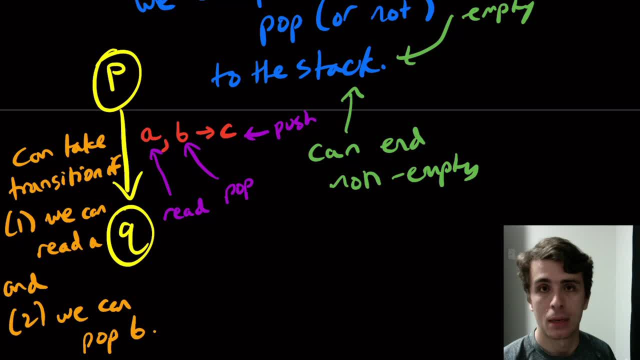 Okay, But all transitions are going to look the same. It's going to look like this, And if I wanted to have a transition that that didn't touch the stack at all, then I would just set B and C, both to be epsilon.